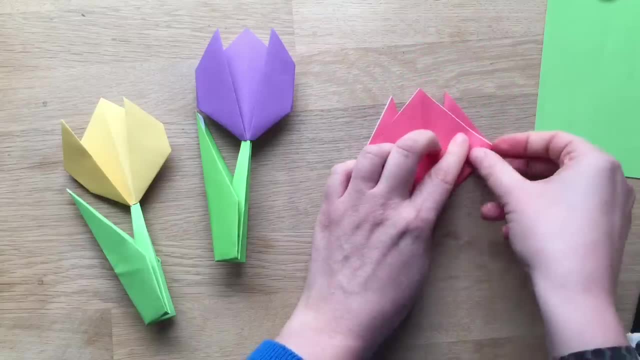 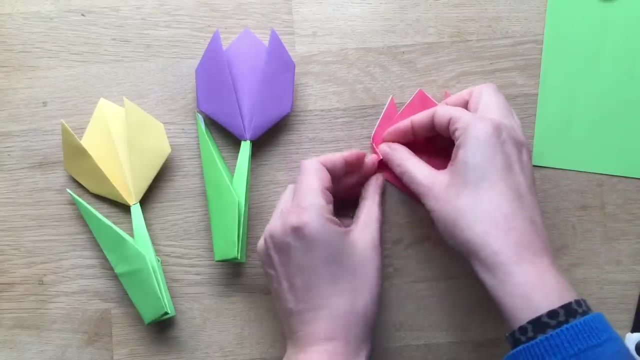 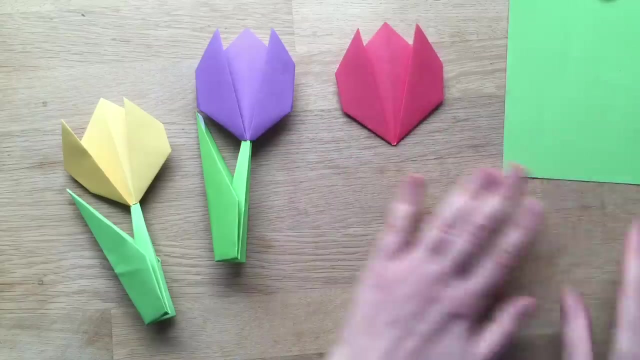 around and you just tuck the corners in. I'm going to fold this like so and fold this like so Now. if you wish, you can fold this in half and then fold it in half. You can stick this onto a card and draw the rest of your flower, or you can keep. 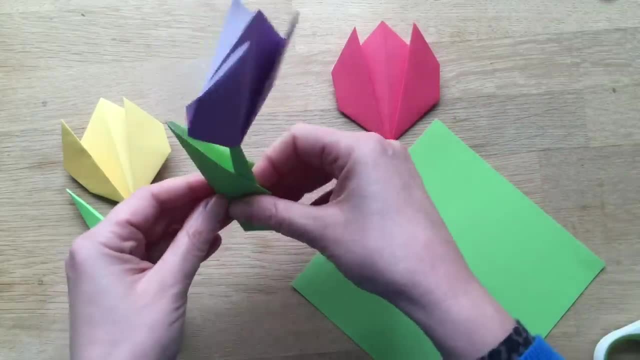 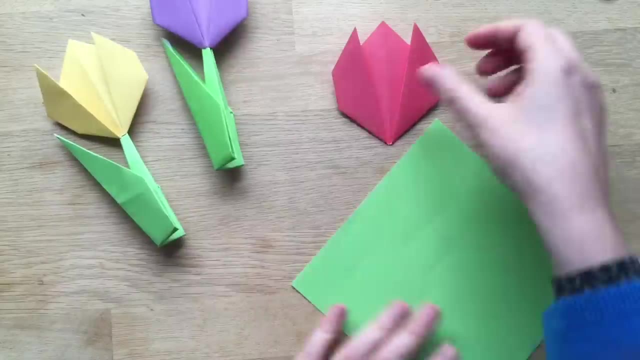 watching and see how we make the stem, And the stem, if I'm doing it right, will actually stand up like that. So to do the stem again, you need this time 15 centimetres by 15 centimetres. I'm going to turn it around so you have the. 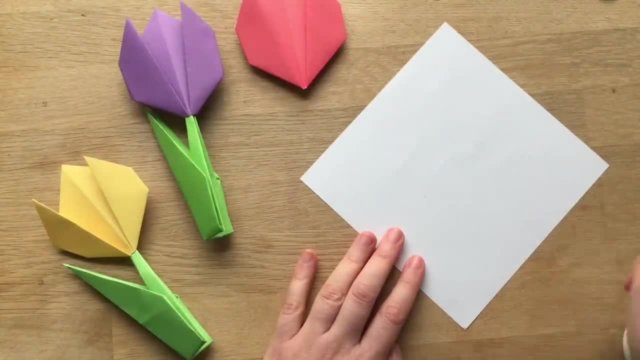 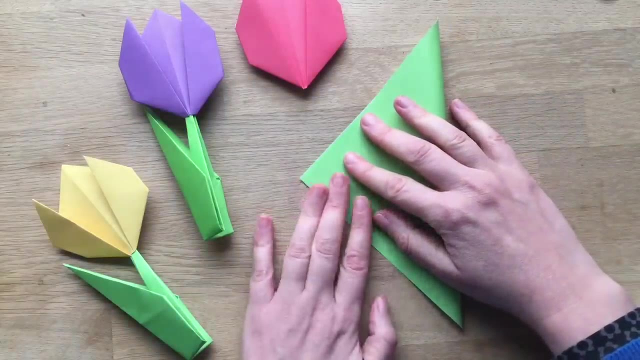 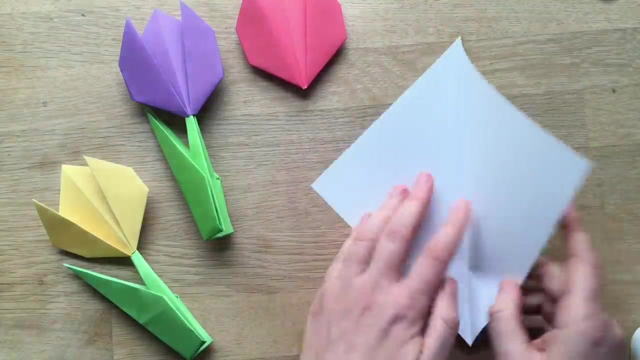 diagonal. Take that side to this side. Actually, it doesn't really matter. You can do it the other way as well, because it is a square and it just means you have to turn your paper around. The main thing is you're going to end up with another triangle. This time you open it up and now. 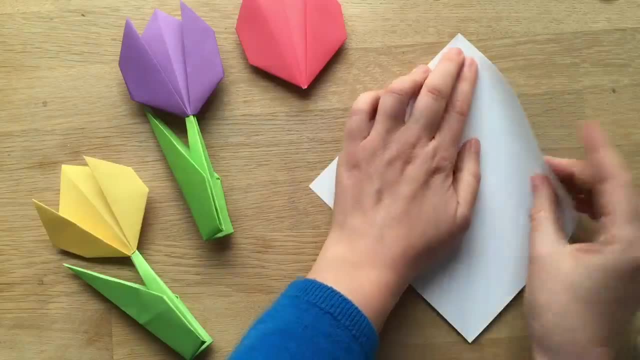 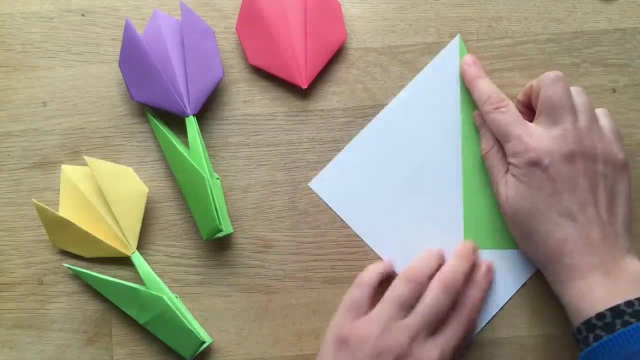 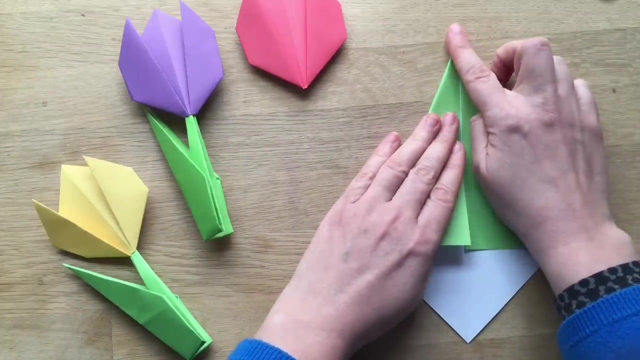 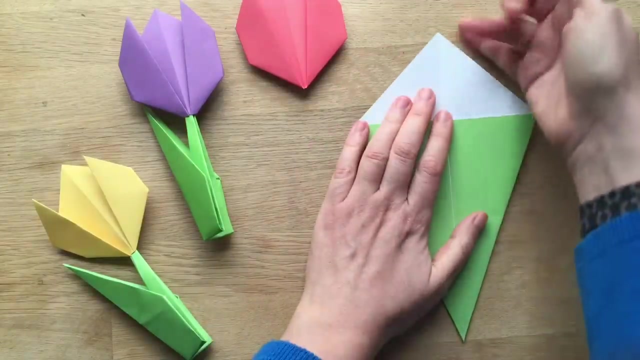 you bring this edge into the centre. So now you bring that edge again into the centre. so you've got like a kite. Try and do this as needs as you possibly can, especially at the tip. Now, to make it easy, I'm going to turn it round and again I'm going to bring this side in. 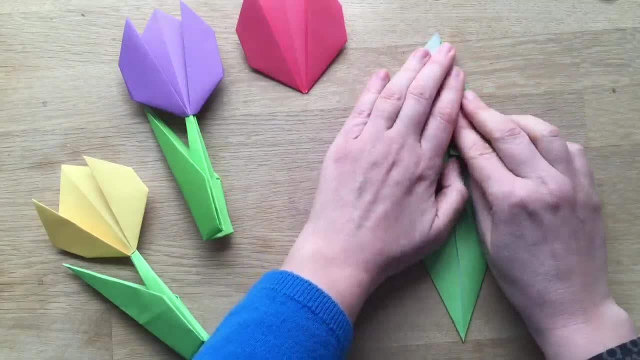 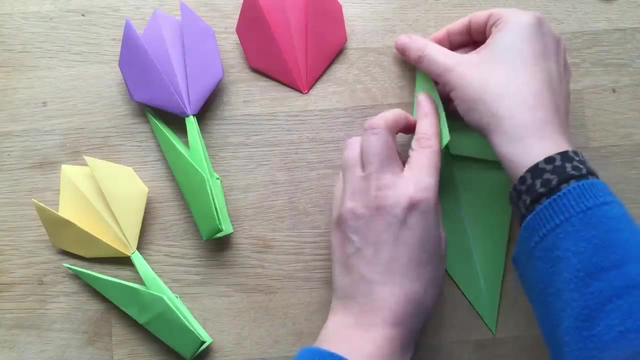 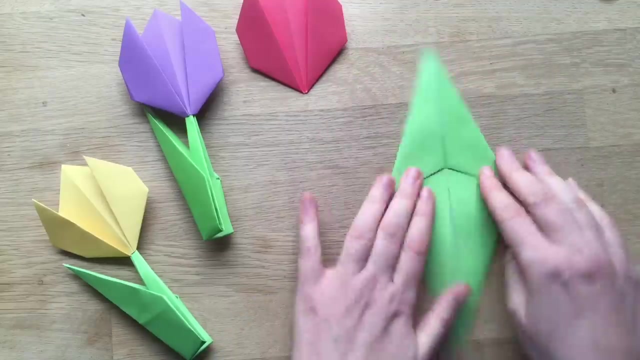 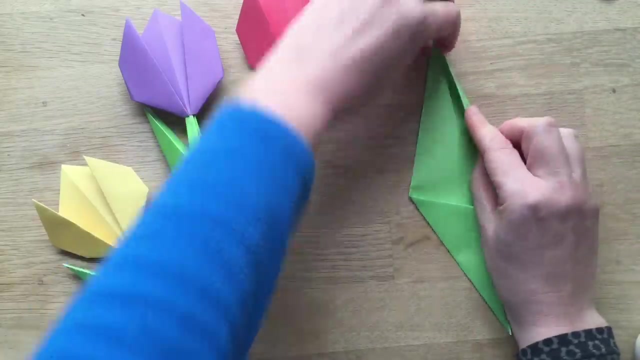 like so, and then I'm going to bring this side in, Alright, so Ok, now I'm going to turn it around again and bring this side in again. so that's the first one. you did the one, the side you did first. you're going to fold in a second time. 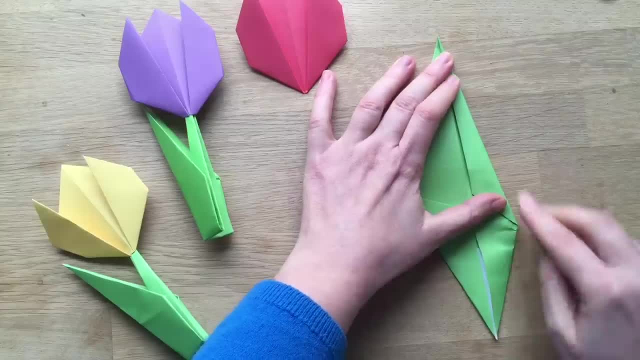 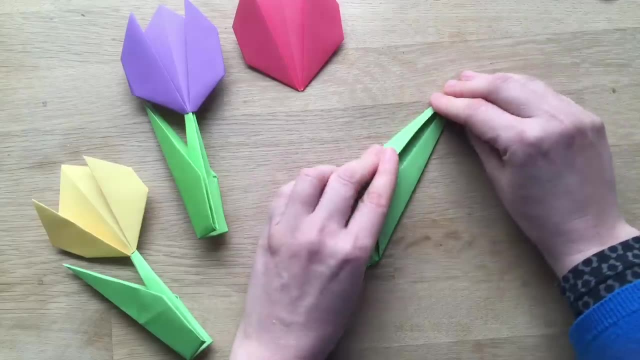 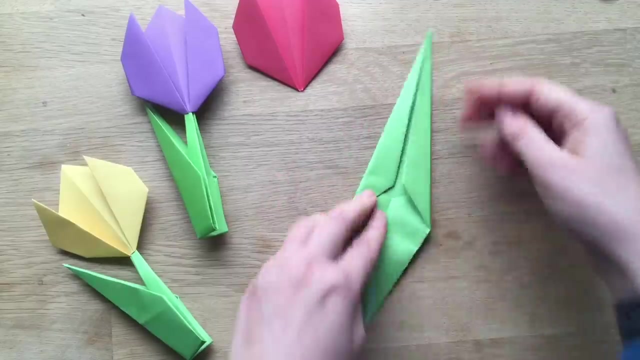 there we go. so this is where you have to fold really carefully and neatly, because it does get a little bit stiff and again same on this side you can bring it in like so okay, so now you've got a really nice long, thin bit and then a little fatter bit. bring the thin bit, the top tip, all the.